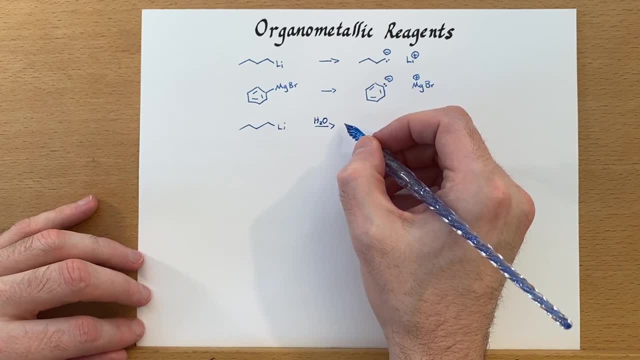 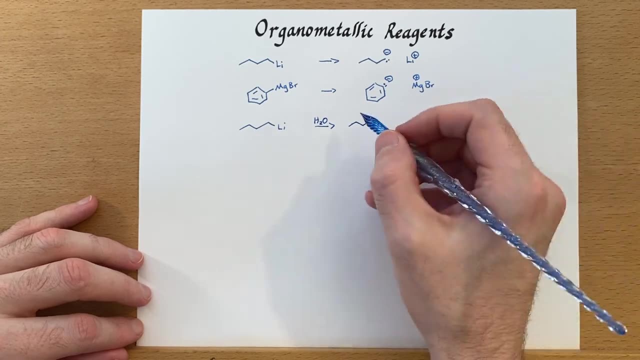 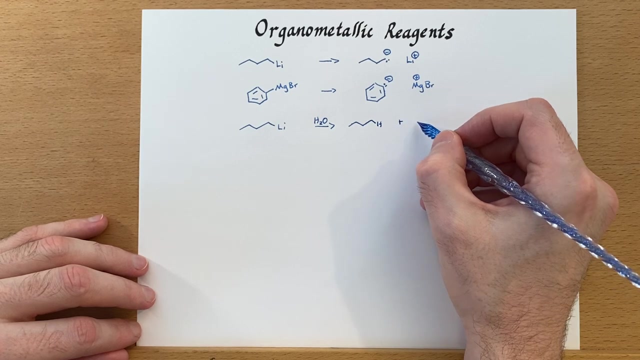 so if it has a chance it's exposed to air, it tends to catch on fire, And, of course, butane is in your little cigarette lighters typically, and and so you'll end up with a situation on your hands and when it's reacting with water. 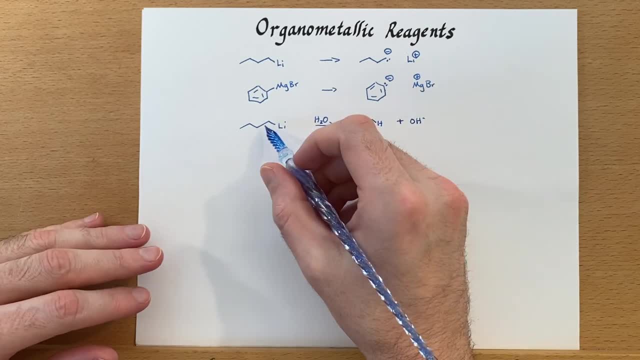 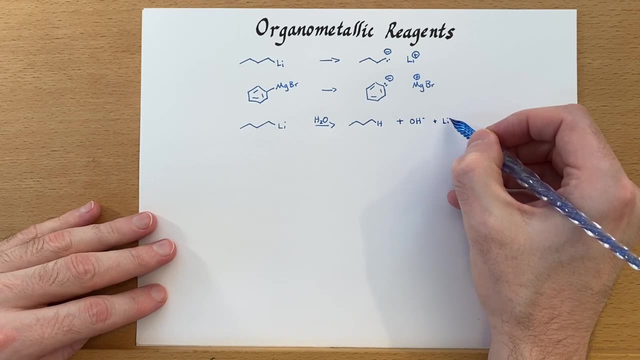 in the air or anywhere. this type of reaction is quite exothermic, so it can just start on fire like that. I guess the point here is: just make sure we're not using a lot of oxygen, because if we're not using a lot of oxygen then we're not. 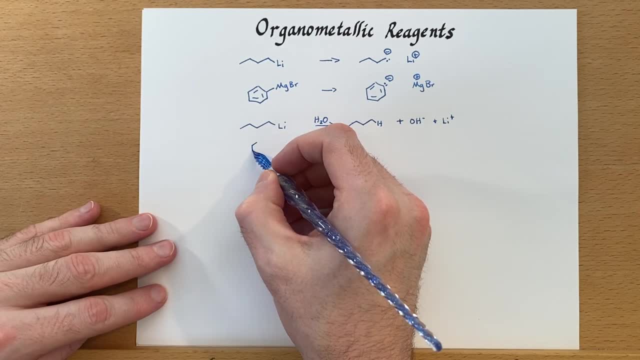 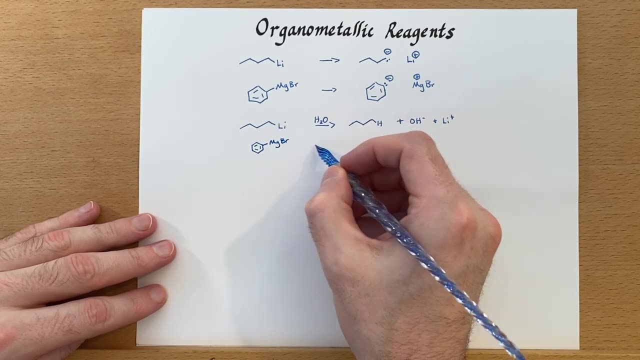 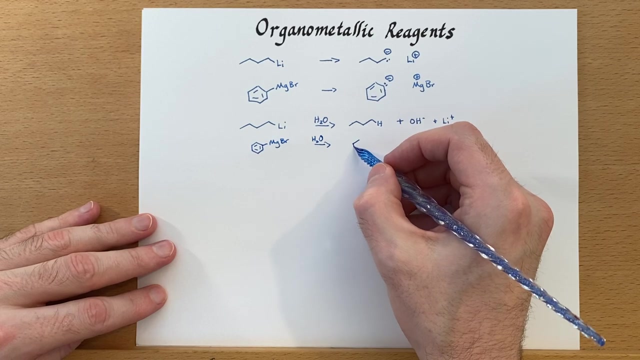 going to be able to produce a lot of oxygen. So if we're not using a lot of oxygen, we're not using protic solvents when we're trying to use these organometallic reagents. This really is a terrible scenario. just adding water to these. 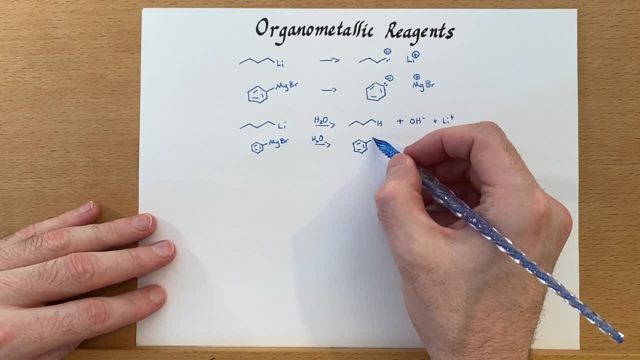 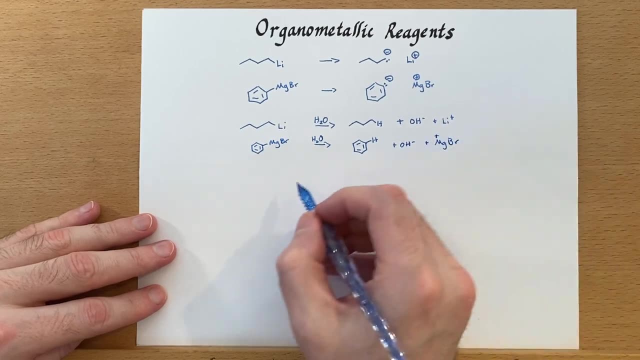 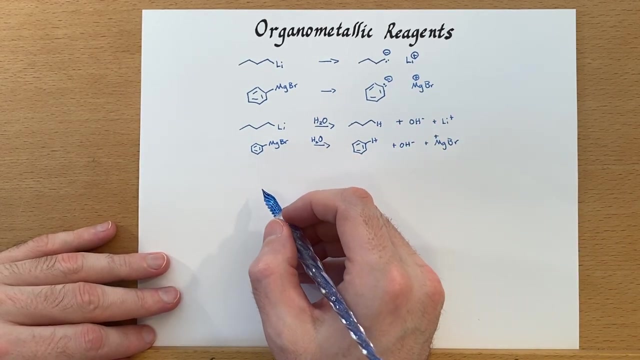 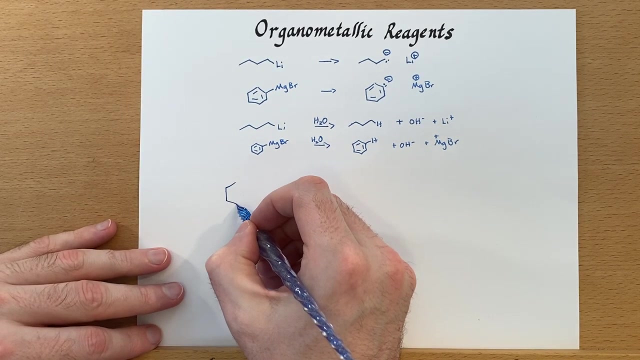 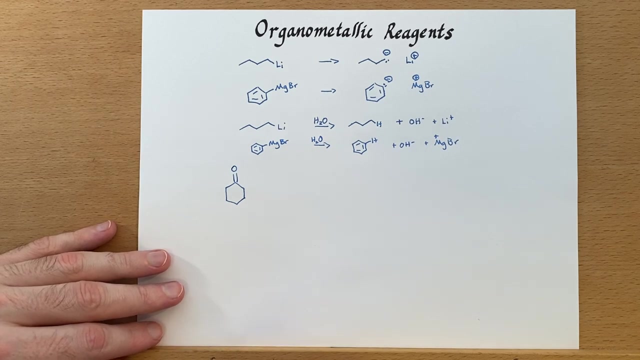 reagents, You will very, very quickly destroy them Now. these are quite useful, though, because they will attack ketones and aldehydes and some of these other reagents, so let's just look at one of those reactions. Actually, we'll look at a couple. So we've got cyclohexanone, and we'll just go ahead. 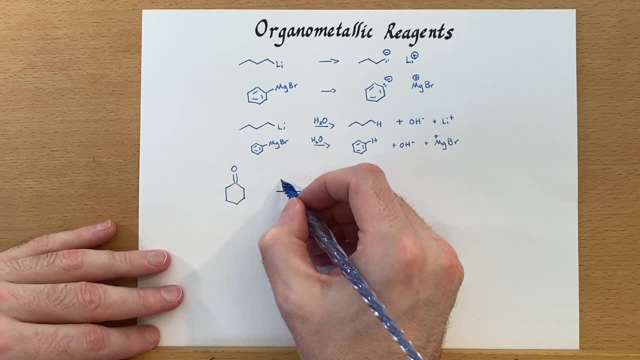 and attack the reactions. The first reaction is a excuses ft examination. So if we want to test this reaction with fucking oxygen, we'll have to shoot oxygen up in the air. this with an organolithium reagent. I'm going to use ethyl lithium and we'll have to do this in 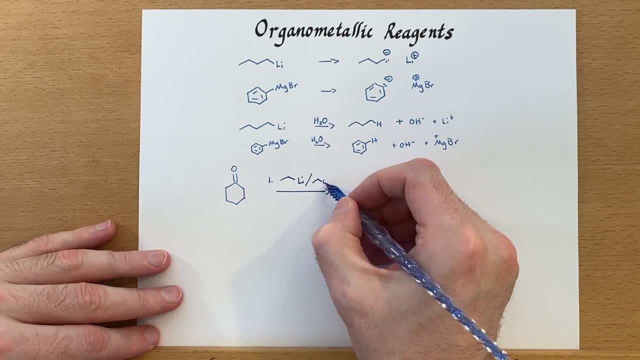 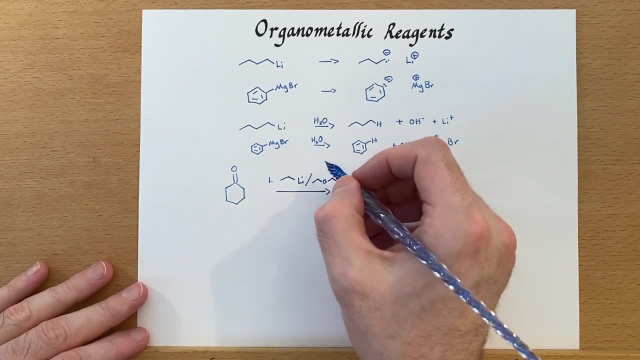 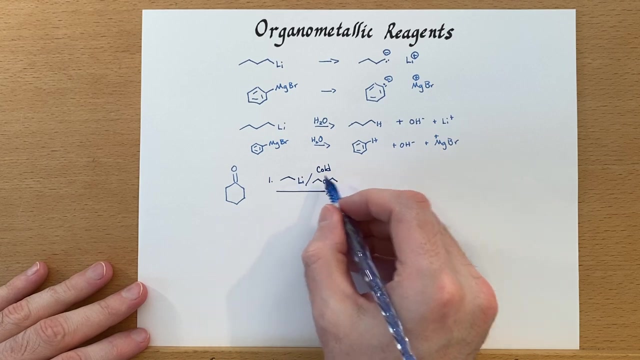 one step here. We'll use diethyl ether, which is typically the reagents that you'd want to use with these organometallics. It's usually some kind of ether and we're going to run this reaction in a cold temperature because this is a very aggressive. 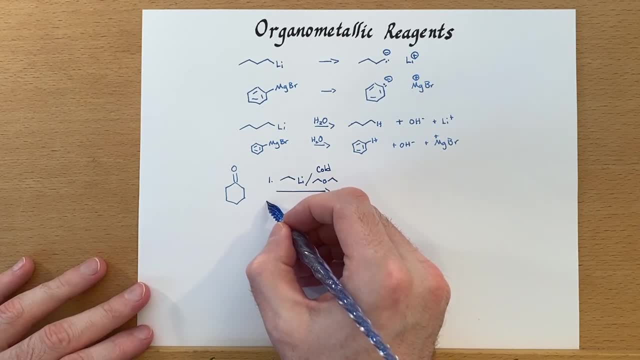 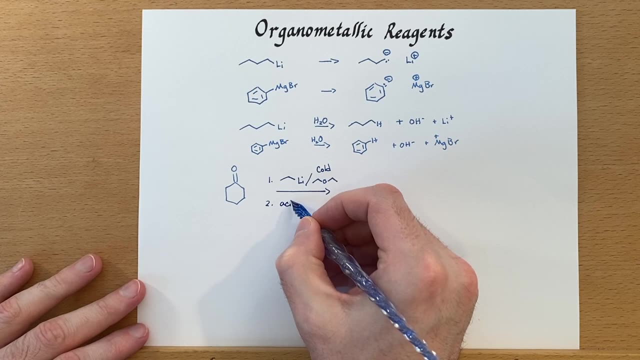 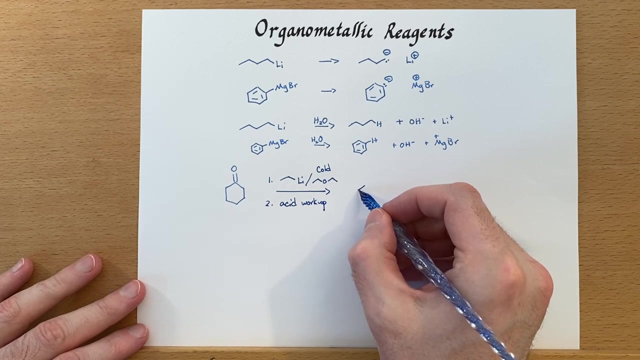 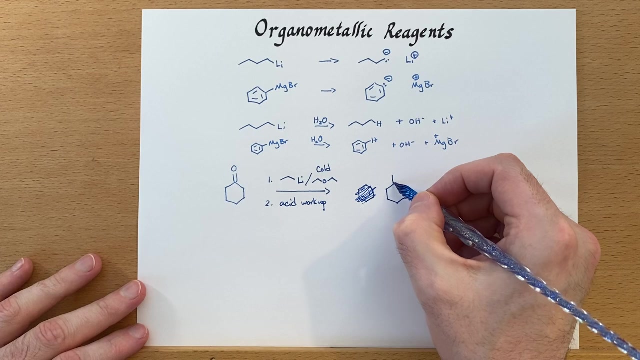 reagent here. The lithium is powerful stuff and after we do that reaction we'll need a little acid workup just to get the proton on the oxygen. Oh well, that's not what I want to talk about there. I'm sure we've all done that. 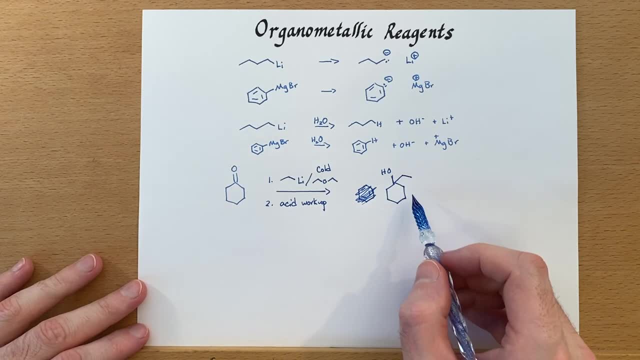 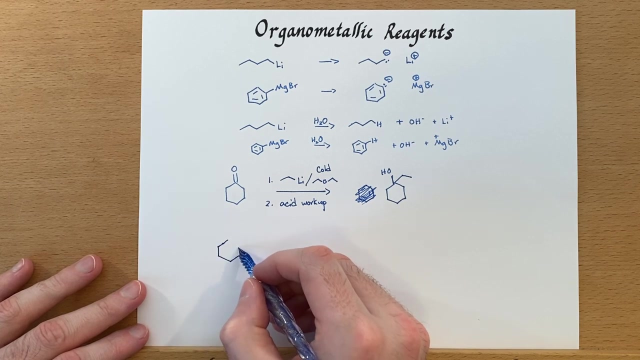 All right. so here we've got our substituted alcohol on the cyclohexane, not the benzene ring. So we've got the alcohol here and we've added our organolithium or ethyl group on. All right, let's look at another reaction that we could do, this time with a nitrile. 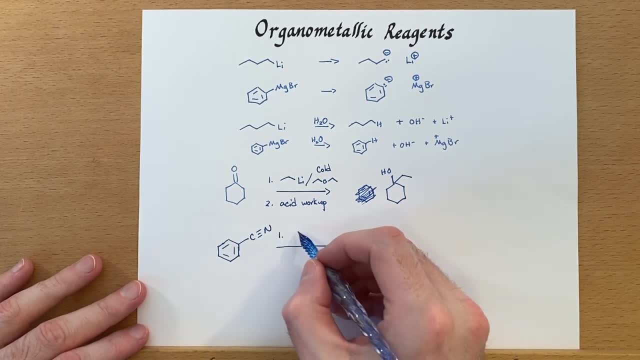 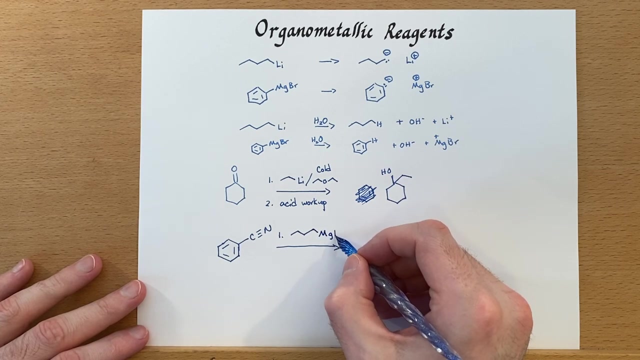 We can change this up to the Grignard reagent Now. this would work with the Grignard reagent as well. So you really get your choice, and I would say that if you can use the Grignard, they're a little easier to work with. They don't catch on fire when they're exposed to air. 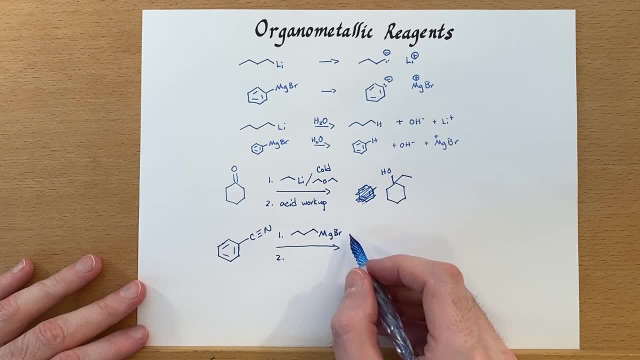 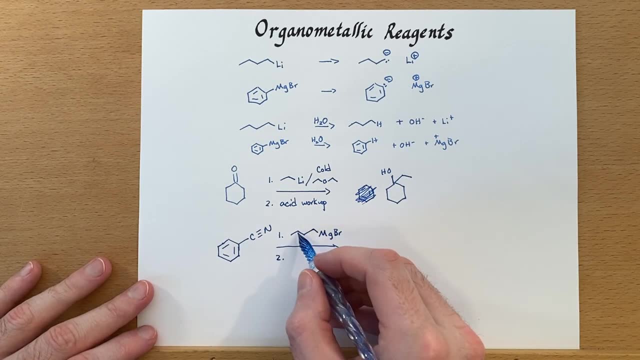 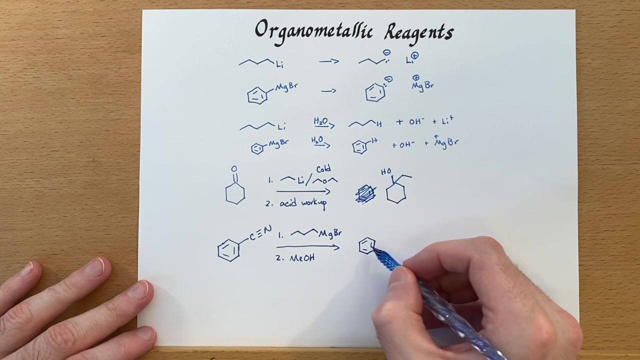 It's just a little bit safer. They're also pretty easy to manufacture. You just need really dry conditions and you just need the corresponding bromine and magnesium metal and that is a typical laboratory that is done in organic chemistry And we're going to do that as well. You'll see a video based on how to do that coming up. 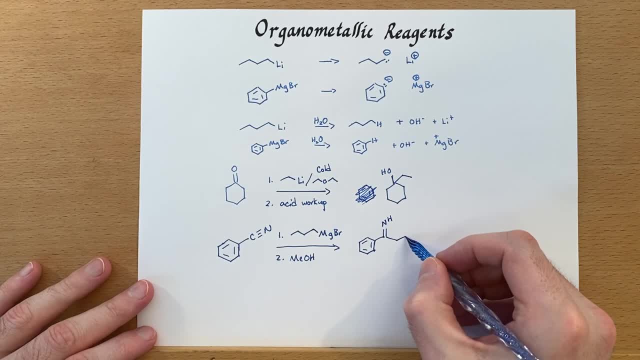 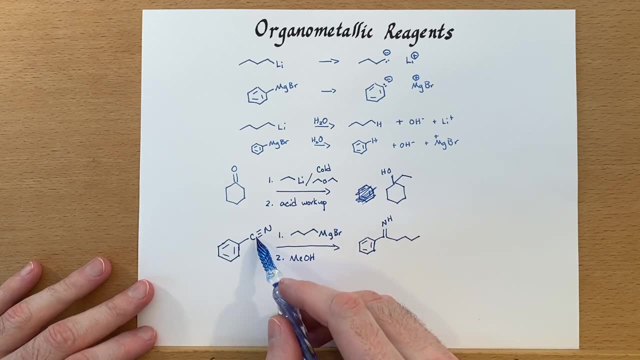 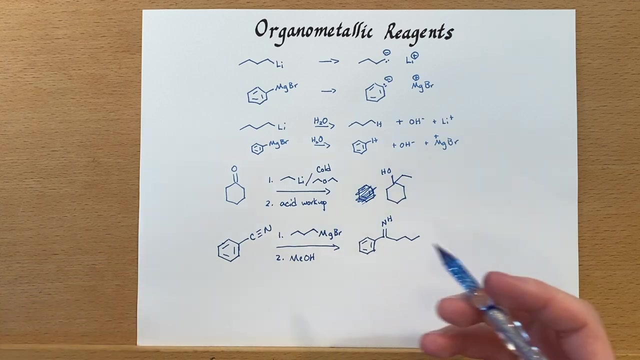 in a few weeks actually. In this case we're going to have the nucleophile come in and then we're going to have the nitrile- One of the electrons goes up here- and then we're going to use the methanol here to go ahead and add that proton on there. Now we could. 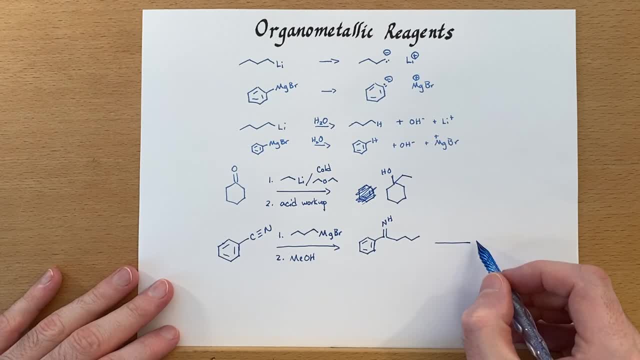 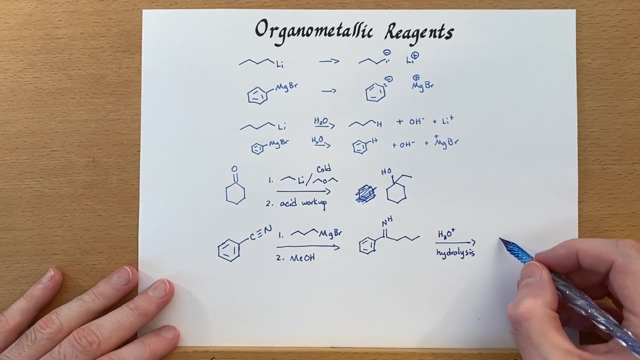 stop right here. or, if we want to, we could hydrolyze the nitrogen and convert it into a ketone Using some acid. So if we want the ketone, that's a way to end up with one, And we can also choose whatever we want for the R group on this side. Now, within reason,